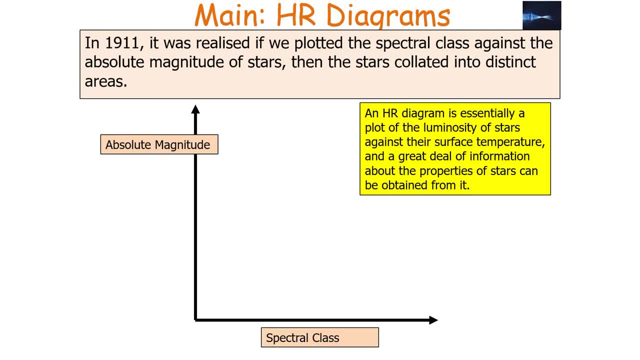 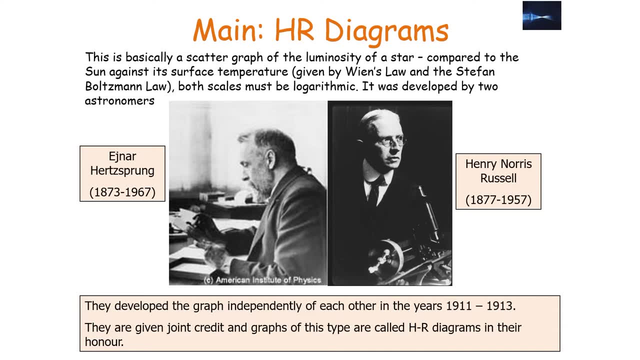 and a great deal of information about the products of the stars can be obtained from it. So this is a scatter graph of the luminosity of a star compared to the sun against its surface temperature, which is worked out by the vine displacement law and the stellar 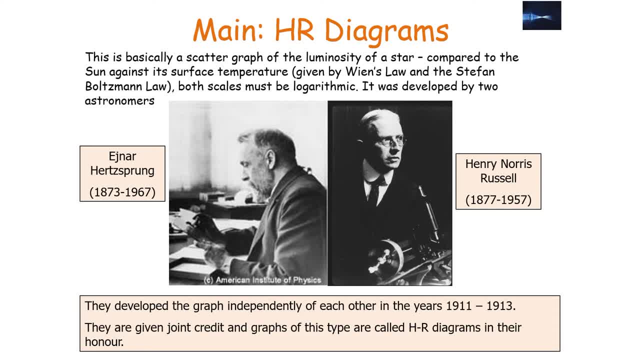 Now both scales are logarithmic and it was developed independently by two separate astronomers, Hertzsprung and Russell. Now they developed the graph independently of each other in the years 1911 to 1913, and they're given joint credit in graphs of this type called Hertzsprung-Russell diagrams, in their honor. 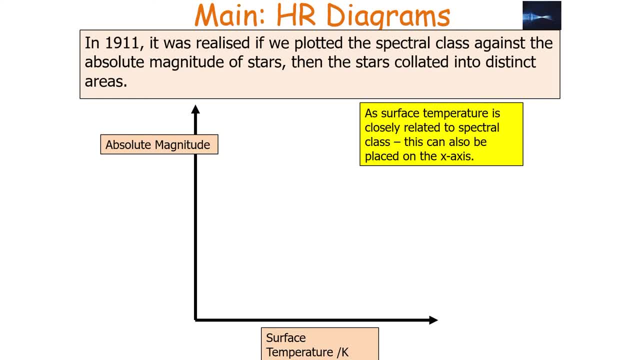 So, as the surface temperature in the star is closely related to the spectral class, we can either place the surface temperature or the spectral class on the x-axis of a Hertzsprung-Russell diagram, whilst the y-axis is a measure of the brightness of a star, its absolute magnitude. 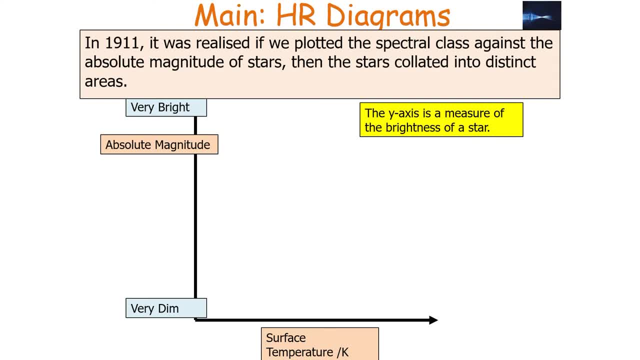 Now, in our scale we have very bright at the top and very dim at the bottom. Now what we know from absolute magnitude tells us that very bright is a very negative value, whilst very dim is a very positive value. so we've got to remember the magnitude scale system. 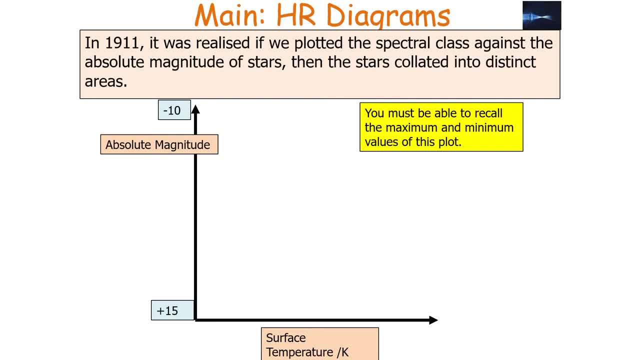 Now you've got to be able to recall the maximum and minimum values of this plot for a standard Hertzsprung-Russell diagram. Now, a standard Hertzsprung-Russell diagram is a very positive value, and a standard Hertzsprung-Russell diagram goes from plus 15 at the dimmest to minus 10 at the most brightest. 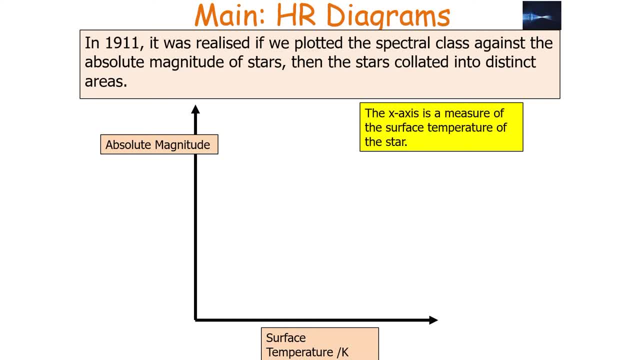 Now, the x-axis is a measure of the surface temperature of the star. Once again, we have very hot at the left-hand side and we have very cool at the right-hand side. So we tend to find that it's 50,000 Kelvin at the left-hand side, whilst it's 2,500 Kelvin at the right-hand side. 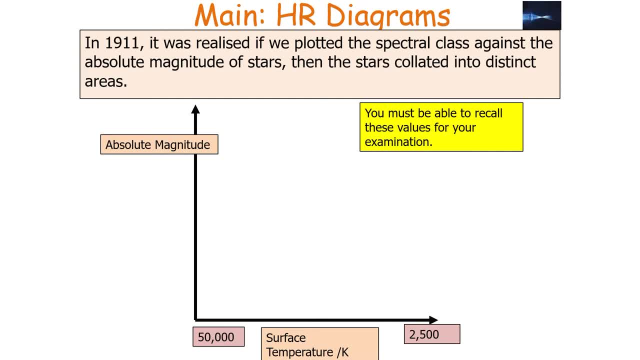 Now you have to be able to recall these values for your examination. Now, just to note, this scale is non-linear And just to clarify, we've got very hot on the left-hand side of our Hertzsprung-Russell diagram. 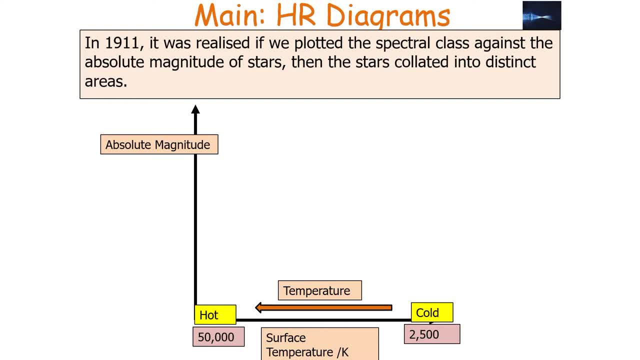 and very cold on the right-hand side. So our temperature goes to the left-hand side of the diagram, so it increases the further left you go. So the temperature is scaled in the opposite direction to what you expect from most other graphs in science. 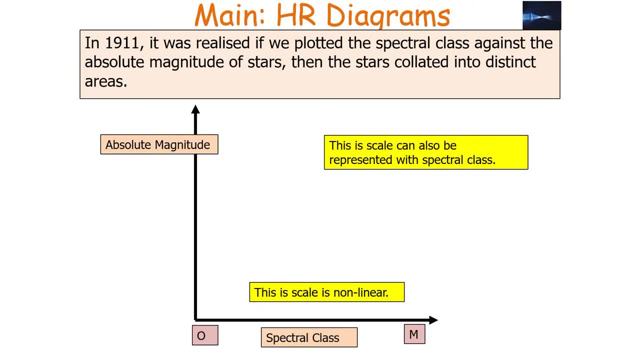 Now this scale, whilst it is non-linear, can also be represented with a spectral class, with O on the left-hand side and M on the right-hand side, So this leads to the graph in the foreground. So what we're going to do is we're going to divide that by the following areas: 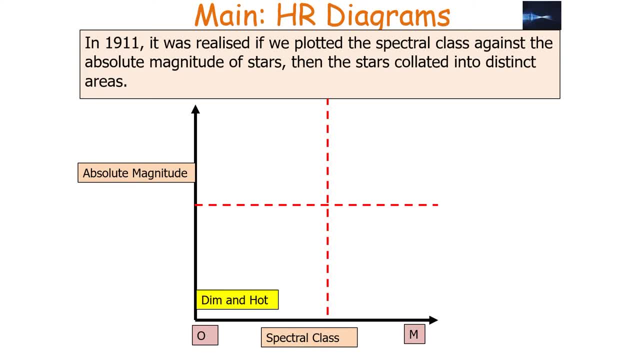 In the top left-hand corner of your Hertzsprung-Russell diagram, you get bright and hot stars. In the bottom left-hand corner of your Hertzsprung-Russell diagram, we get hot and dim stars. In the top right-hand corner, we get the bright and cool stars. 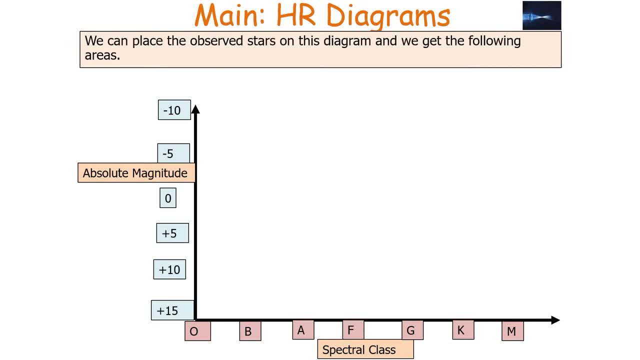 And we get the dim and cool stars in the bottom right-hand corner. So we can place the observed stars on this diagram and we get the following areas. So just to clarify, we'll be separating out our Hertzsprung-Russell diagram. 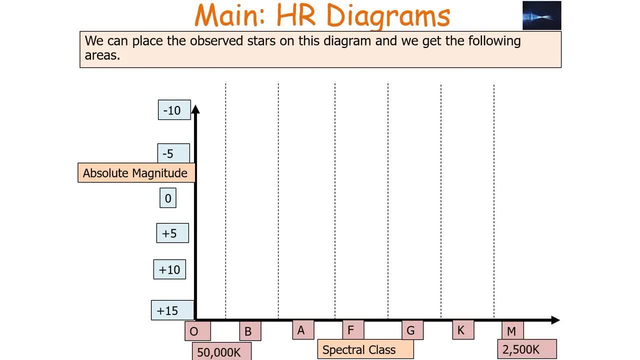 from the spectral classes, or you can consider it in the different temperatures. Now you'll notice that the stars on the Hertzsprung-Russell diagram are not randomly scattered. They are divided into three principal groupings, as you can see here. 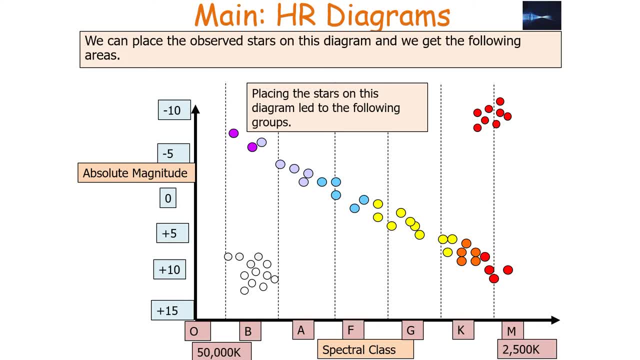 So placing the stars on the Hertzsprung-Russell diagram scale leads to the following groups: Now it can be approximated that all of these stars have roughly the same power output. But we've got the red giants at the top right-hand corner. 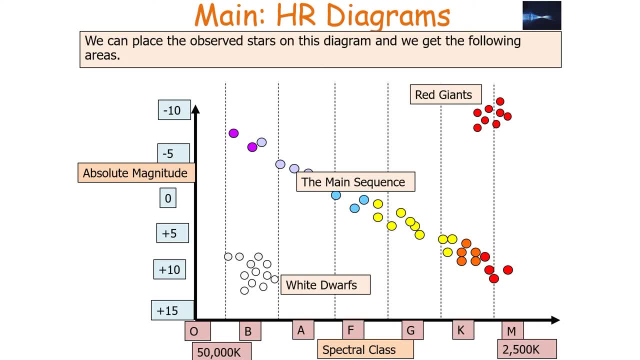 the main sequence, in the band in the middle and the white dwarfs at the bottom left-hand corner. Now let us consider the main sequence first. Now you've got to be able to place two stars in the main sequence. The first one is our own Sun, which has an absolute magnitude of plus five. 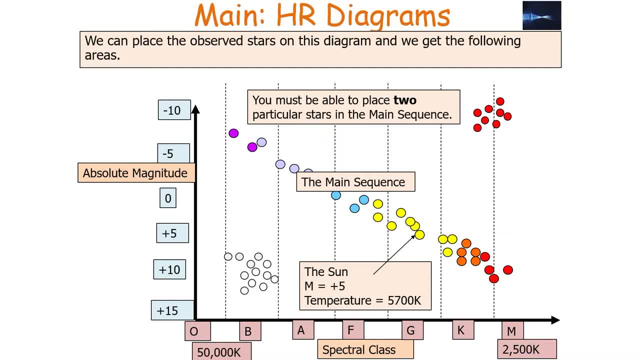 and a surface temperature of 5,700 Kelvin. So it's in the G-type spectral class. And you've also got to consider Vega, which forms the basis of our magnitude system in astronomy. So the absolute magnitude of Vega is approximately plus five and it has 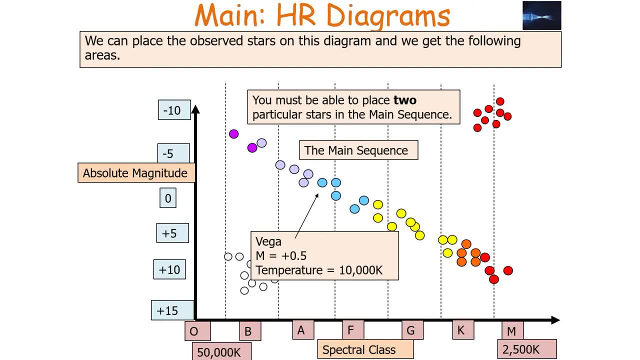 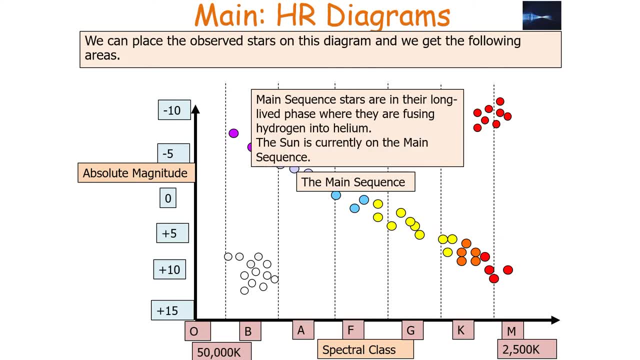 a surface temperature of 10,000 Kelvin, so it's in the A-spectral class. Now main sequence stars are in their long-lived phase, where they're fusing hydrogen into helium. Now our Sun is currently on its main sequence. 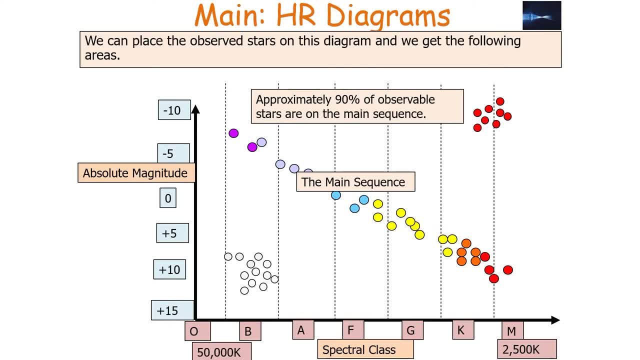 Now, approximately 90% of observable stars in our universe are currently on the main sequence. Now, at the top of the main sequence are the hot and luminous blue stars. At the bottom are the cool and dim reddish stars. Now you've also got the red giant. 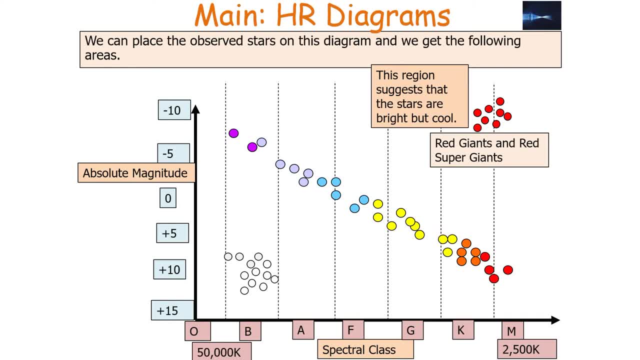 and supergiant group. Now this region suggests that the stars are bright, but they're quite cool. Now you've got to be able to recognize one star from this region, which is Betelgeuse. Now Betelgeuse again has an absolute magnitude of approximately. 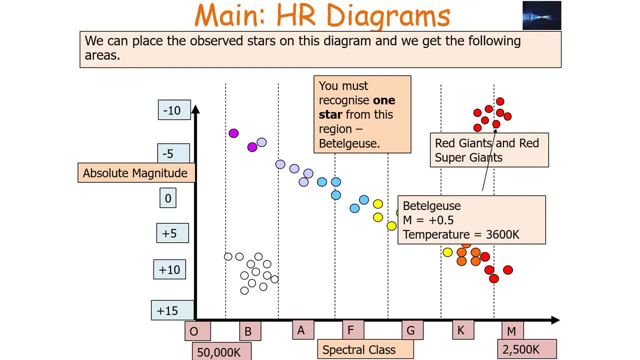 minus five and then has a temperature of 3,700 Kelvin. So as a result, belongs in that part of your Hertzsprung-Russell diagram. Now we know that P equals sigma A, t to the four. So the red color suggests a low. 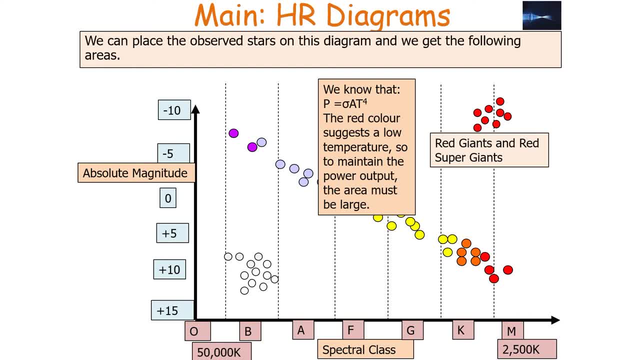 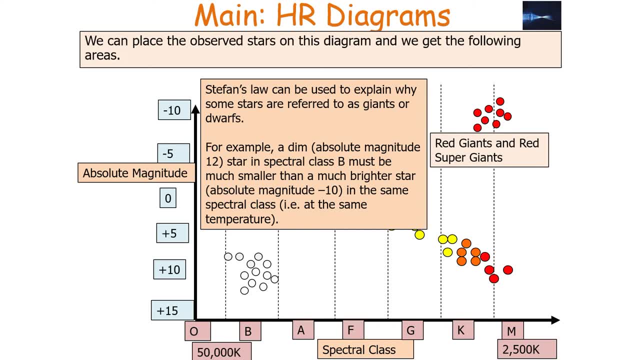 temperature, so to maintain the power output, the area of these particular stars must be large. So this tells us that Stefan's law can be used to explain why some stars are referred to as giants or some stars referred to as dwarfs. So, for example, a dim star with an absolute 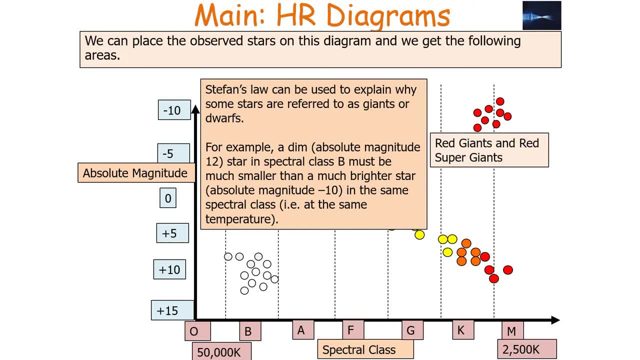 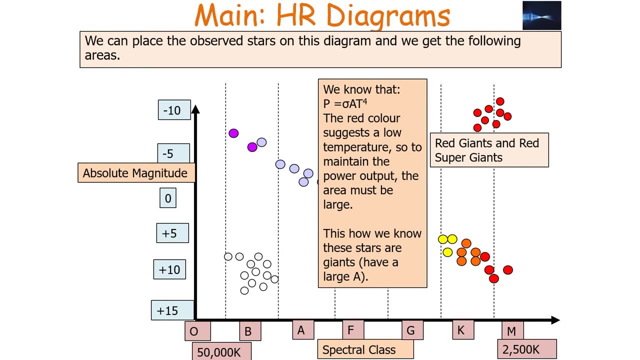 magnitude of plus 10 in spectral class B must be much smaller than the much brighter star absolute magnitude minus 10 in the same spectral class. So it allows you to work out the sizes of our different stars. Now, because we know that P equals sigma A, t to the four, 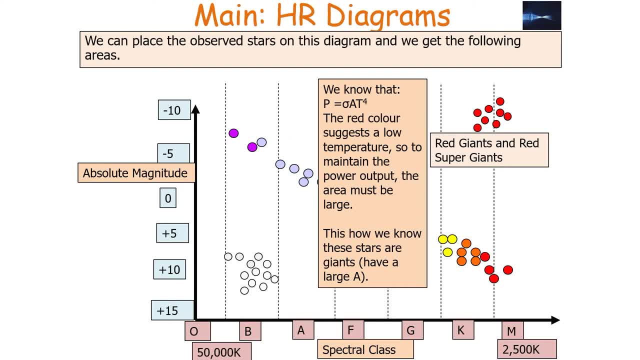 we know that these stars must be giant because the low temperature indicates that to maintain the power output, the area must be large. Now the red giants are the stars which have moved off the main sequence and the fusion reactions other than hydrogen to helium are happening inside of them. 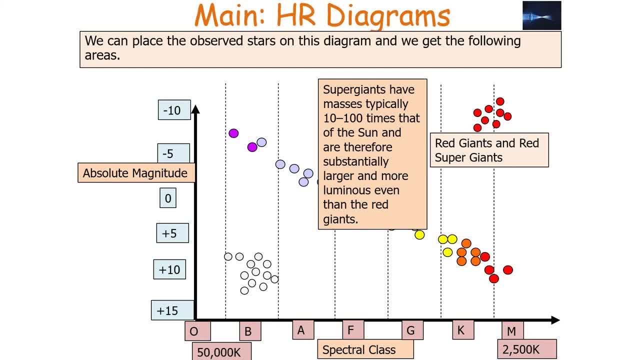 Now supergiants have masses as masses typically 10 to 100 times that of the sun, and are therefore substantially larger and much more luminous than even the red giants. Now supergiants are hot enough for nuclear fusion reactions to produce carbon and the heavier elements. 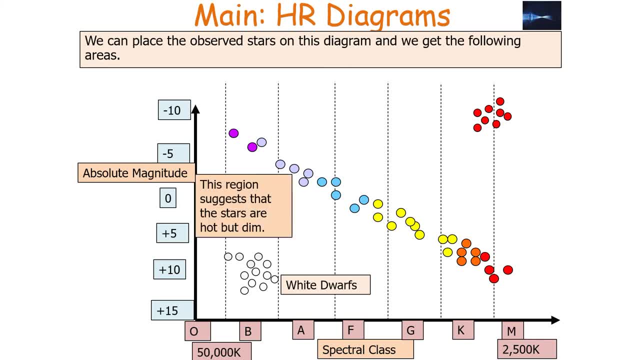 Now the final group we need to focus on are the white dwarfs. Now, this region suggests that the stars here are hot but dim. Now we know that P equals sigma A, t to the four, So the white colour suggests a high temperature. 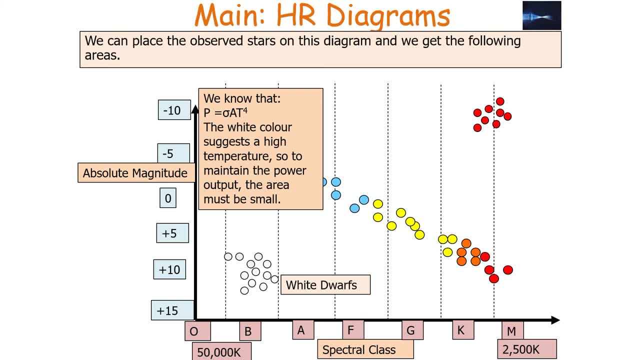 So to maintain the power output, the area of our star must be quite small. So the white colour is very important because it indicates that these stars must be small dwarfs and have a small surface area to them. Now, white dwarfs are stars at the end of their lives, where all the fusion reactions 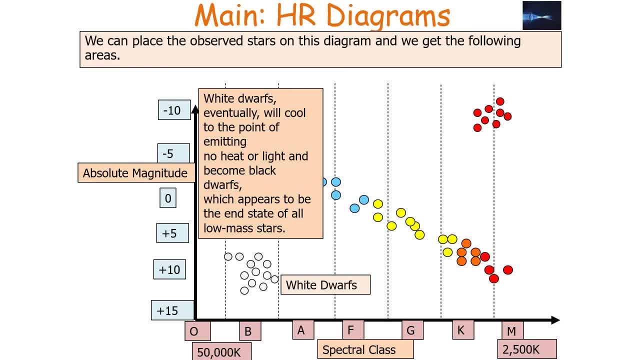 have stopped and they are slowly cooling down. Now white dwarfs will eventually cool to the point of emitting no heat or no light or no radiation and become black dwarfs, which appears to be the end state of all low mass stars. Now the significance of the Hertzsprung-Russell. 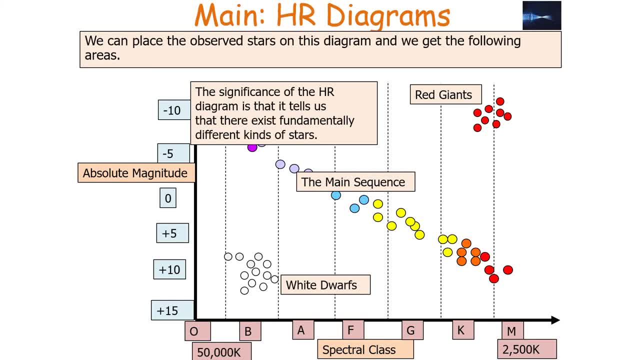 diagram is that it tells us that they exist, that they're fundamentally are different kinds of stars. So when astronomers first saw these groups, they were puzzled: Why were the three distinct types of stars? Well, it was later realised that the stars were at different stages of their life. 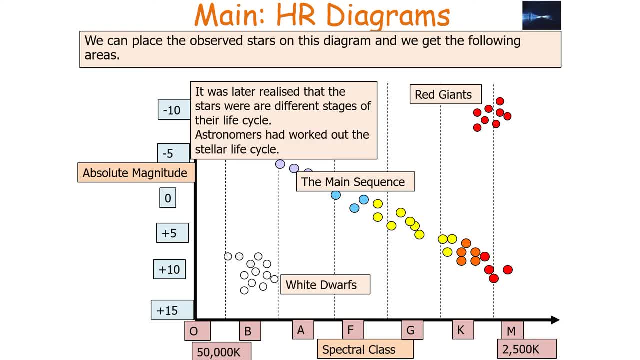 cycle. so it allowed astronomers to work out that there was a stellar life cycle. Now, from the Hertzsprung-Russell diagram we can see different stages of stellar evolution: how stars are born, how they grow old and how they eventually die. 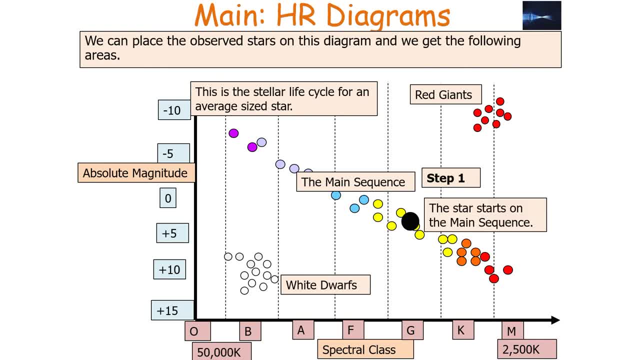 So this is the stellar life cycle for an average sized star. Step one: the star starts on the main sequence. Now the placement of the star on the sequence depends on its size. Now, as the star carries out fusion, it moves along on the main sequence ever so slightly. 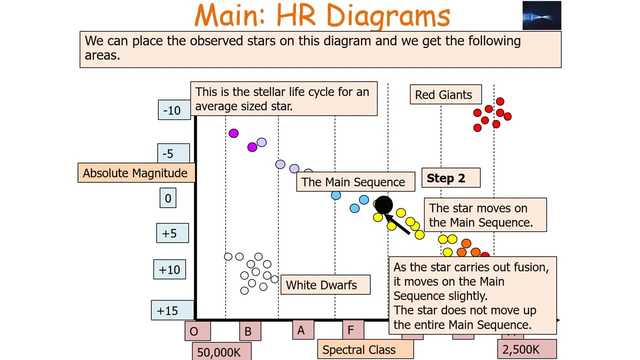 Now the star will not move up the entire main sequence. It won't go from the bottom right to the top left. It might shift a small amount on that main sequence diagonal band but it won't move across all of it. Then the star will become a red giant and move across to our red giant section here. 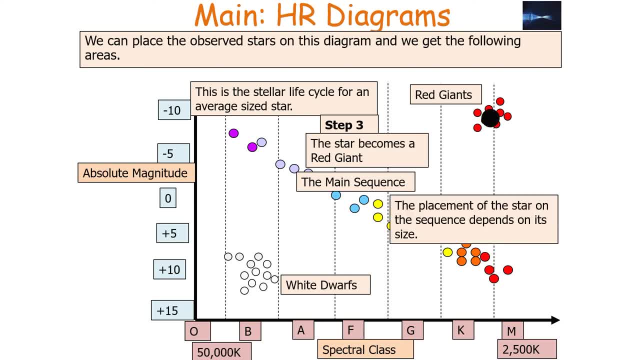 Now, again, the placement of the star on the sequence is dependent on its size. And then finally, in step four, the star becomes a white dwarf, And again the placement of the star on the sequence depends on its size. So you can see here our different stages. 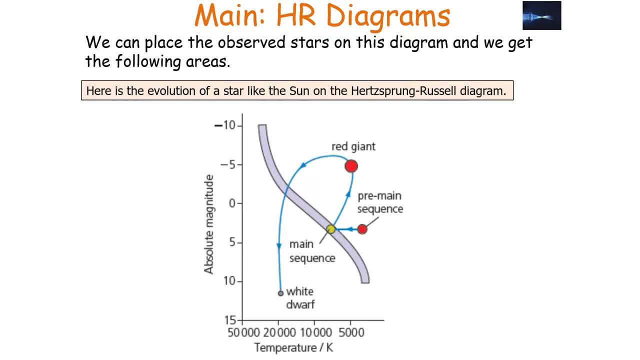 of our stellar evolution for an average sized star. So you can see here a bit more clearly the evolution of a star like the Sun on the Hertzsprung-Russell diagram. Now just to clarify: the Hertzsprung-Russell diagram we cover in AQA, A-Level Physics is a slight 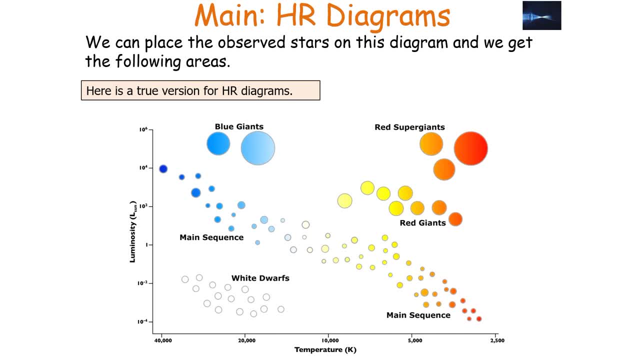 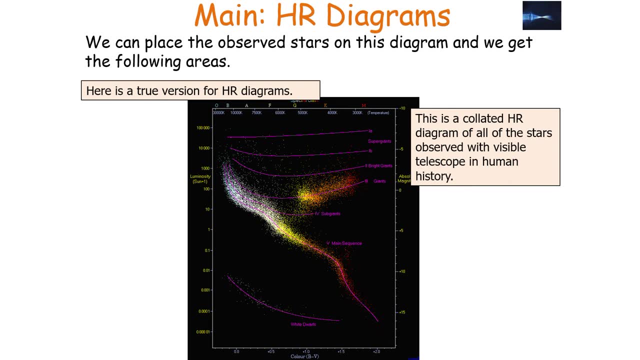 simplification. You can see a more thorough version of the Hertzsprung-Russell diagram, And this, in fact, is a lovely image. It's a collated Hertzsprung-Russell diagram of all of the stars observed.